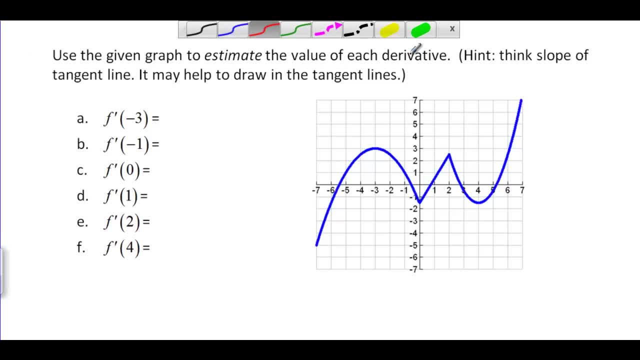 The first derivative it asks us to find. the first slope is the slope of the tangent line at negative 3.. Here's negative 3. I draw in a tangent line here and if I draw it well, it looks like it should be nice. and 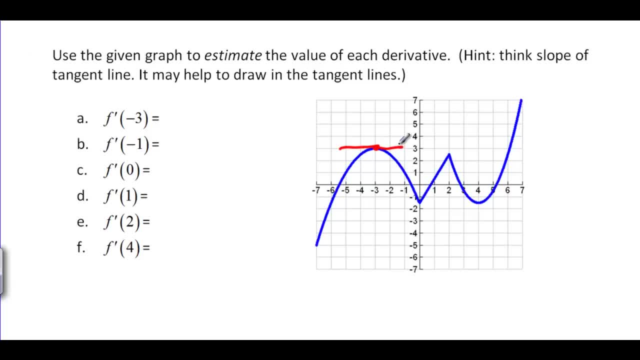 flat. It's the top of the hill there. Anytime you have the top of a hill or the bottom of a hill, like over here at 4,, you're going to have a slope of 0.. Next it asks us to find the slope at negative 1.. 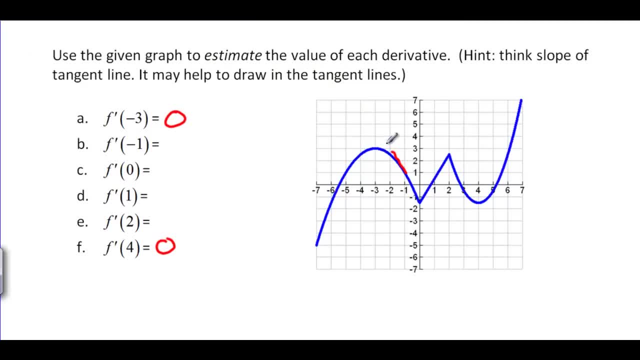 At negative 1, right here. if we draw in a tangent line here, it's harder to be sure, but it looks like the tangent line looks something like this, If I pick some points on this line to look at: here is negative 1,, 1,, and then here's: 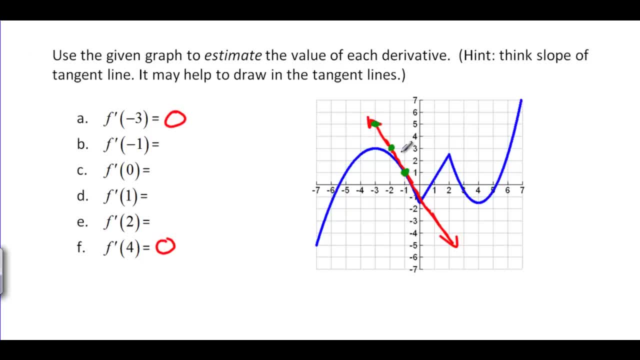 negative 2, 3.. Negative 3, 5.. Negative 3, 5.. Looks like the change in Y is about 2, and the change in X is about 1, so this should be 2 over 1,, which is 2.. 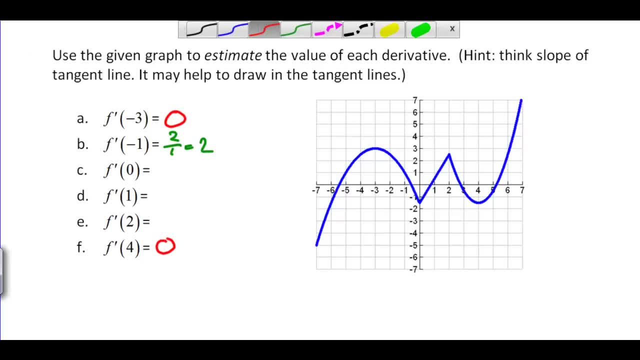 Now, if we look at F prime at 0, here is a very interesting thing, because if I put a point here where X is 0. And I pick any point over here on the right side to estimate the tangent line, it would look like this: 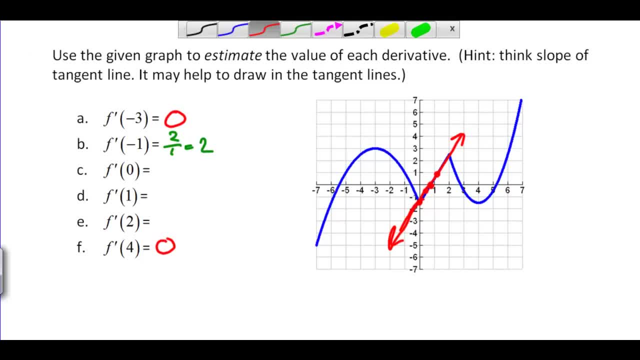 But if I pick any point over here on the left side to estimate the tangent line, it's going to look something like this: As you can see, those slopes are going to disagree. So the limit- Okay, The limit as H goes to 0 from the left side is going to not equal the limit as H goes. 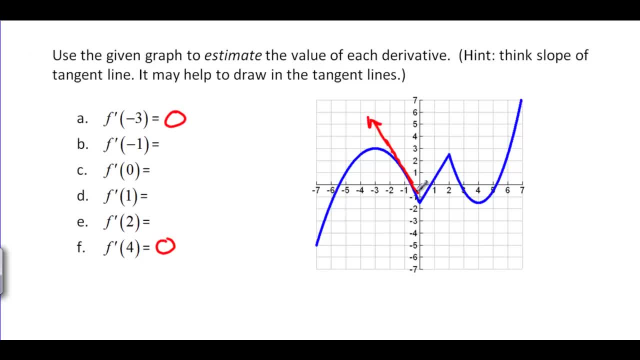 but it looks like the tangent line looks something like this, And if I pick some points on this line to look at, here is negative 1, 1, and then here is negative 2, 1.. Negative 2, 3, and negative 3, 5,. looks like the change in Y is about 2, and the change 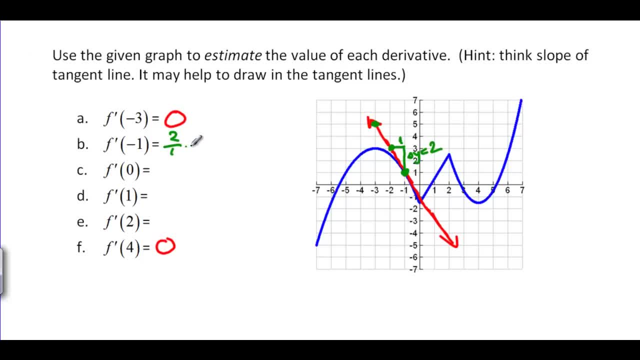 in X is about 1, so this should be 2 over 1, which is 2.. Now if we look at F, prime at 0, here is a very interesting thing, Because if I put a point here where X is 0, and I pick any point over here on the right, 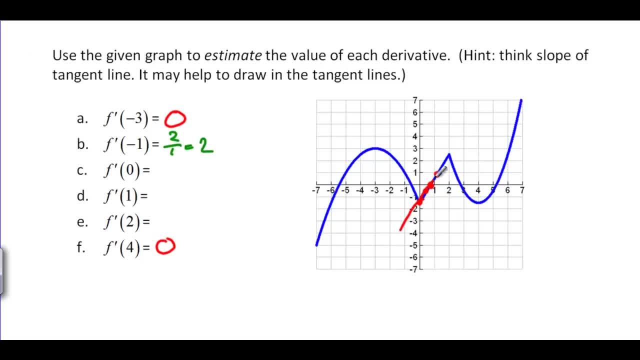 side to estimate the tangent line, it would look like this. but if I pick any point over here on the left side to estimate the tangent line, it's going to look something like this: As you can see, those slopes are going to disagree. 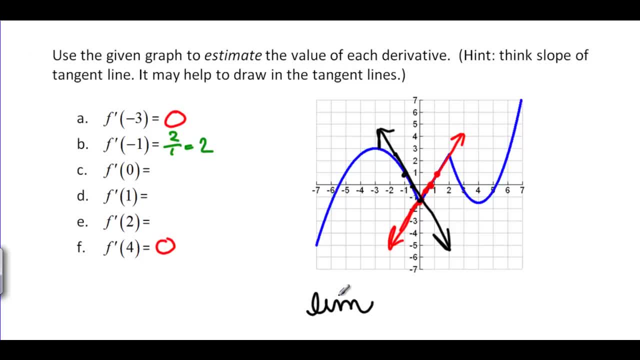 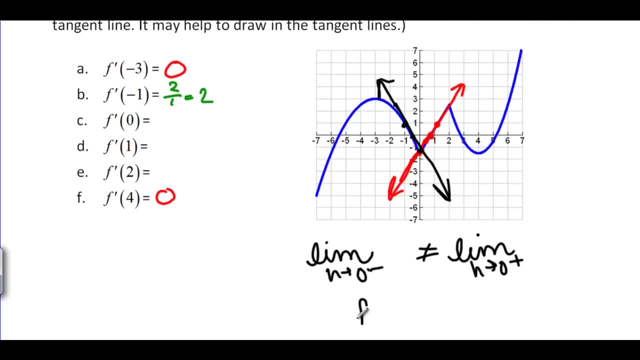 So the limit as H goes to 0 from the left side is going to not equal the limit as H goes to 0 from the right side. We can write this in derivative notation, saying that F prime from the left side at 0 does not equal F prime from the right side at 0.. 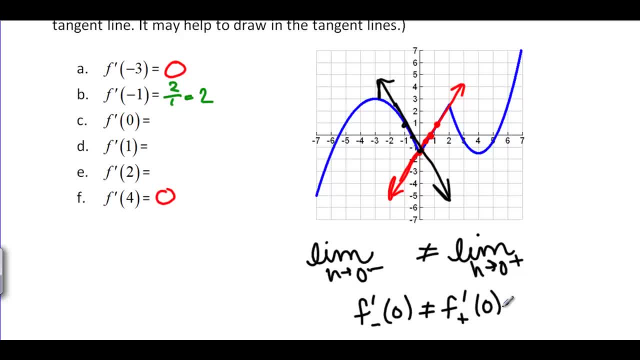 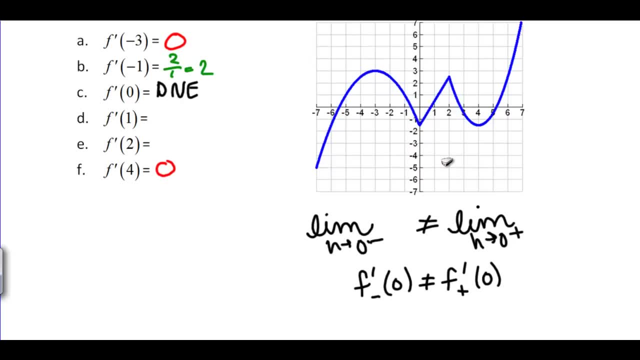 And, just like with our regular limits, this is a limit. so if you get two different answers from the two different sides, then the limit does not exist. Now let's look at F prime of 1.. At 1, our function is actually a straight line, and that means that its tangent line 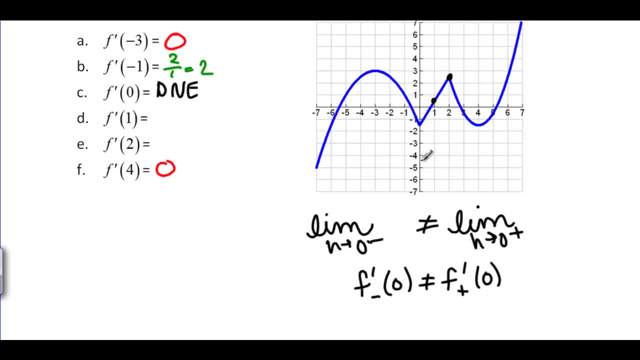 is itself. So if we just pick any two points on this line, at 1 it looks like we're at the point 1, 1 half, And at 2 it looks like we're at the point 2, 2 and a half. 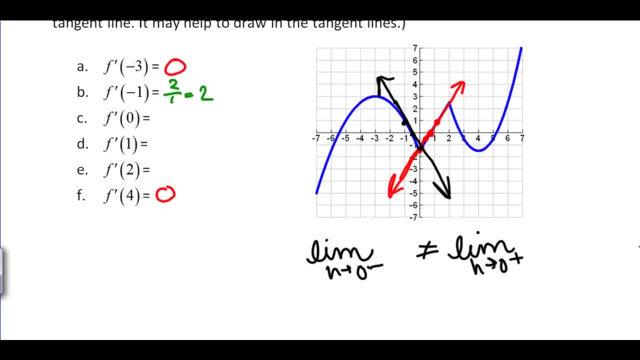 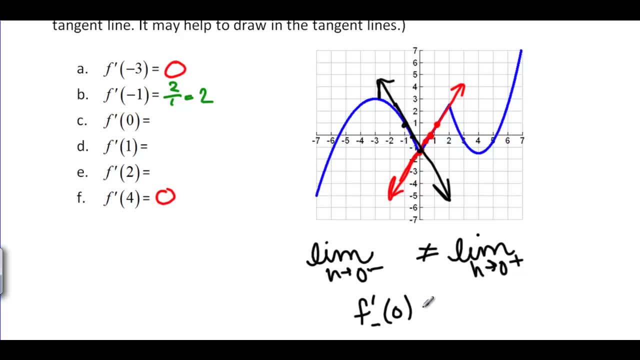 to 0 from the right side. We can write this in derivative notation, saying that F prime from the left side at 0 does not equal F prime from the right side at 0. And, just like with our regular limits, this is a limit. 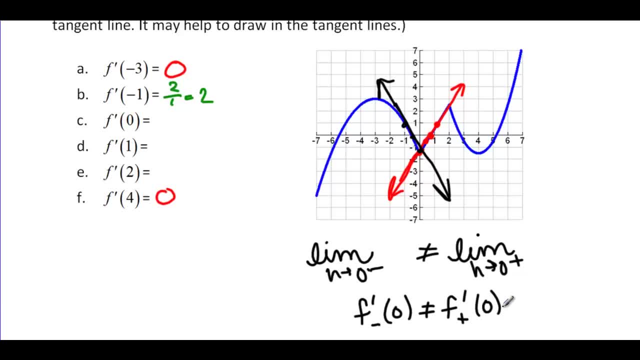 So if you get two different answers, you're going to get a limit. So if you get two different answers, you're going to get a limit. So if you get two different answers from the two different sides, then the limit does not exist. 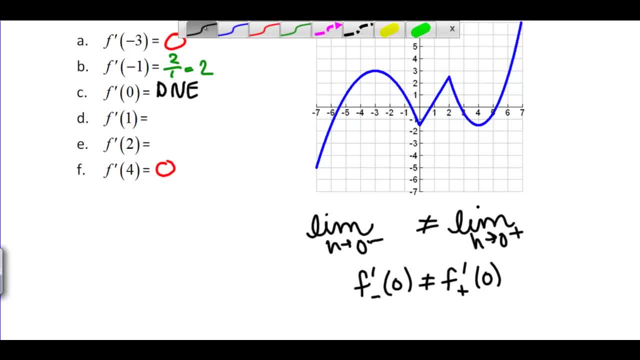 Now let's look at F prime of 1.. At 1, our function is actually a straight line, And that means that its tangent line is itself. So if we just pick any two points on this line at 1, it looks like we're at the point. 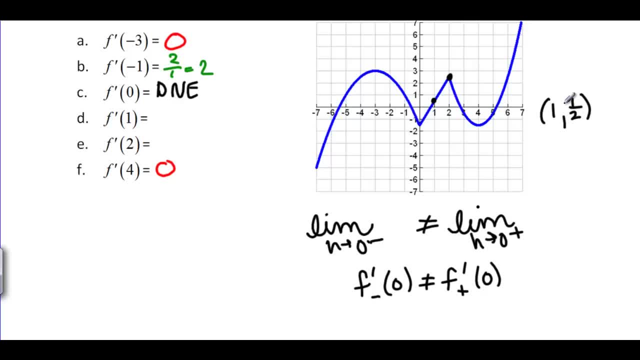 1, 1 half. And at 2, it looks like we're at the point 2, 2.5.. And at 2, it looks like we're at the point 2, 2.5.. And at 1, it looks like we're at the point 1 half. 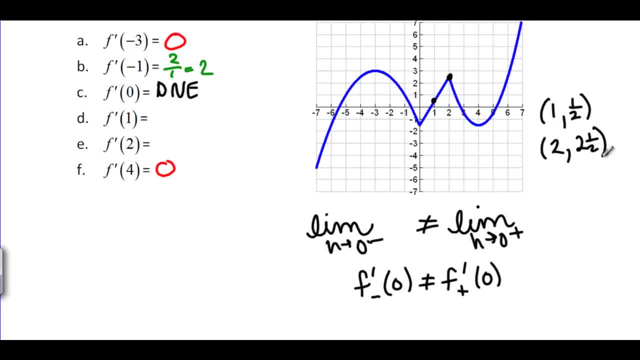 And at 2, it looks like we're at the point 2, 2.5.. 2.5, that would make our change in Y 2 and our change in X 1, so we get 2 over 1, which. 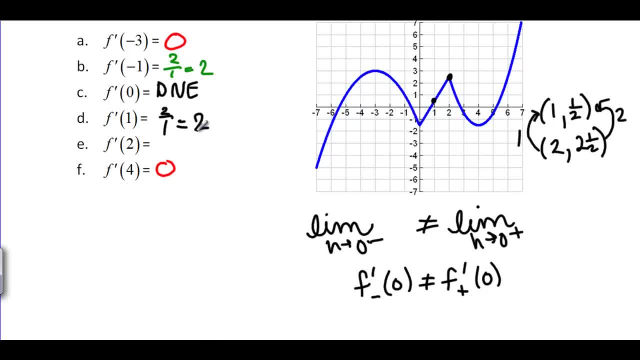 is 2.. Oh, and look, I've realized that we did something wrong back there on F prime of negative 1, because we shouldn't have got the same answer at 1 and at negative 1,, should we? So we have to be careful here. at negative 1, we should have had a point of negative. 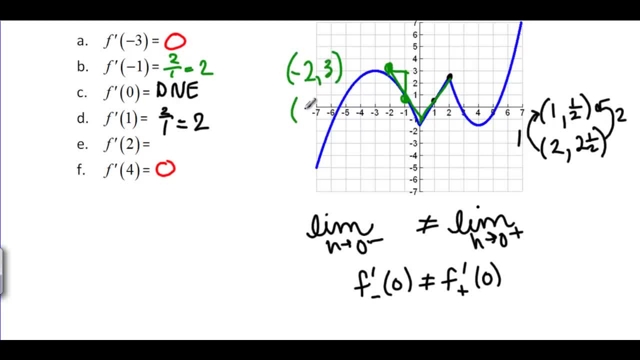 2, 3, and a point of negative 1, 1,. the change in Y here is going: 1 minus 3 is a negative 2, and negative 1 minus 2 is a positive 1, so we should have had negative 2 over 1 to. 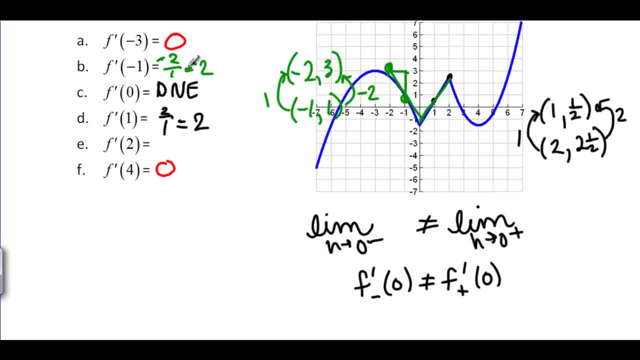 negative 2, actually at negative 1, and that makes sense because, as you can see here, this tangent line is going downhill and should have a negative slope. Alright, we've got one more tangent line to do, and that is F prime of 2, but F prime.